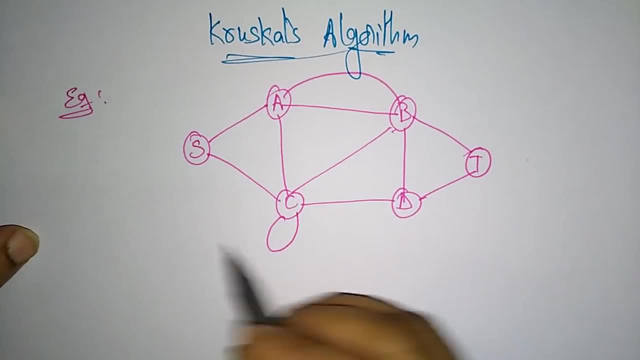 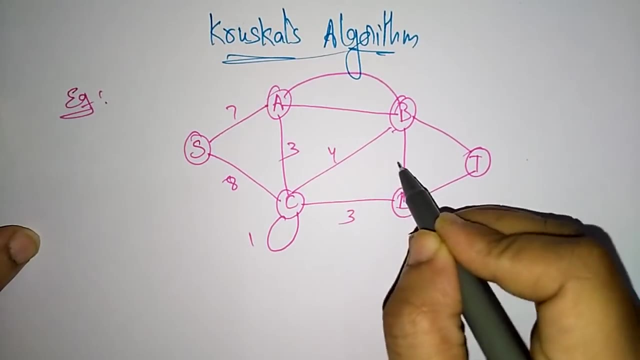 also horrible, and the values for this is eight, seven, three, and the loop is one, three, four, two, five, two, six, Wrong關係, Help me talk some better. ok, Okay, now will take number four and the others and take number five And tercerSorry And. 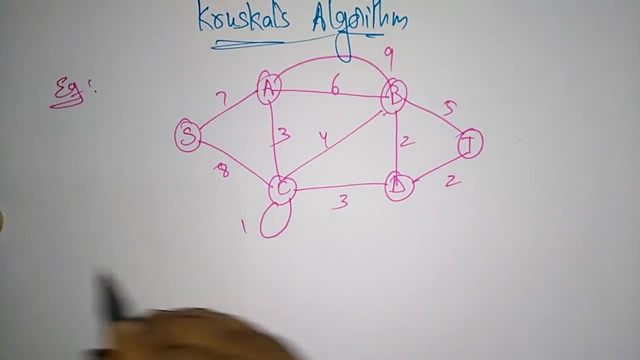 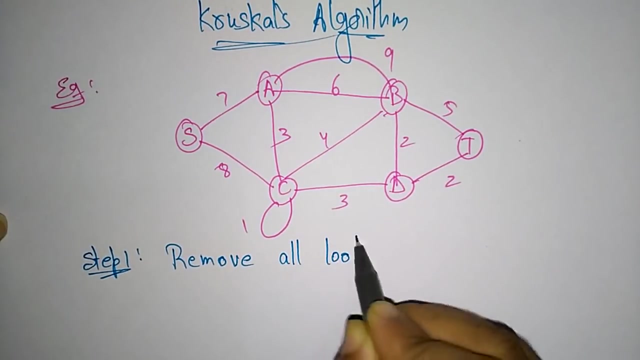 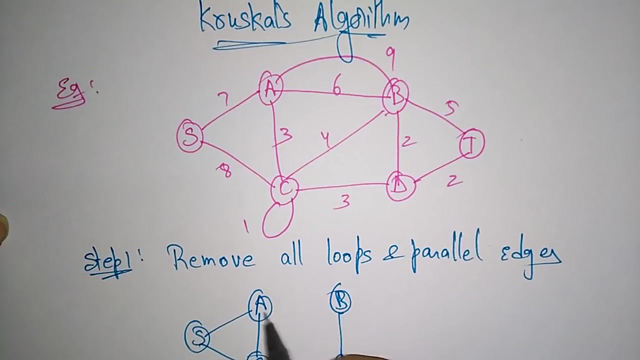 9.. So let's take this as an example. Now coming to the algorithm First step. So in the algorithm, first step is we have to remove all loops and parallel edges. In Krushka's algorithm, first you have to remove all loops and parallel edges. So that means it becomes S, A, C, D, B, T. That's it. 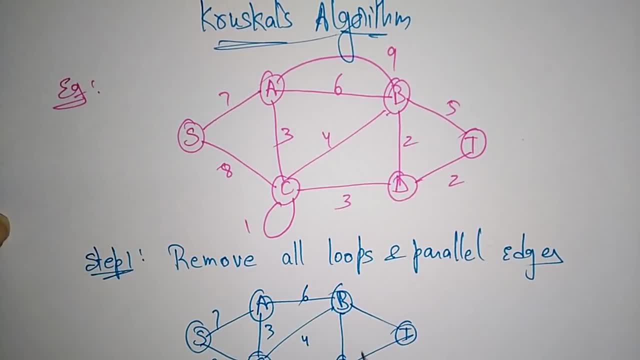 So A 7,, 8,, 3,, 4,, 6,, 3,, 2,, 2,, 5.. So here in this case, if suppose a parallel edge is removed, then we have to remove all loops and parallel edges. So that means it. 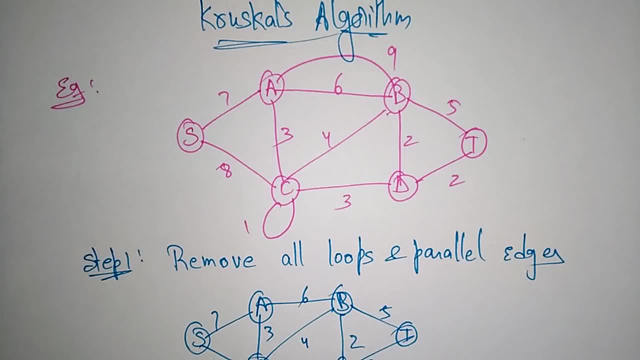 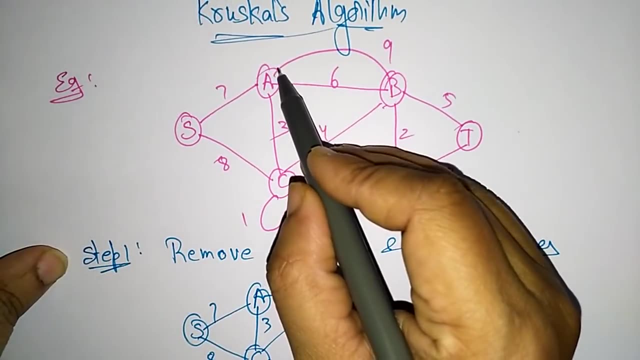 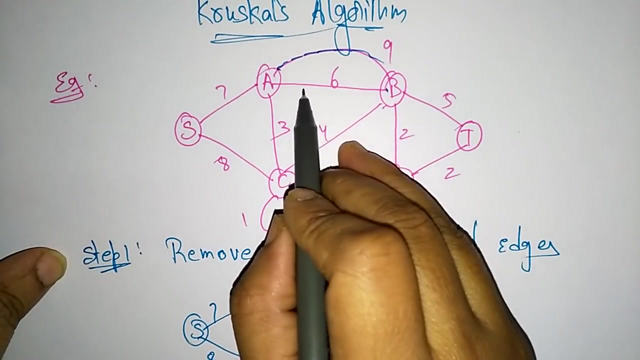 we have to choose the least cost and the remaining all has to be removed. So here the loop I removed and the parallel edge. So this is the parallel edge, So this is parallel edge to this, But here we have to select only the least cost. Instead of selecting 6, I selected 9, because 6 is the least. 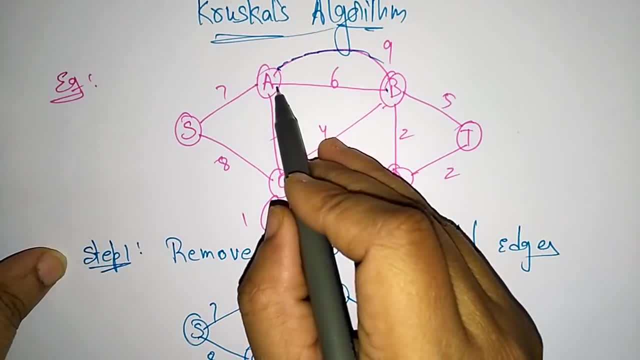 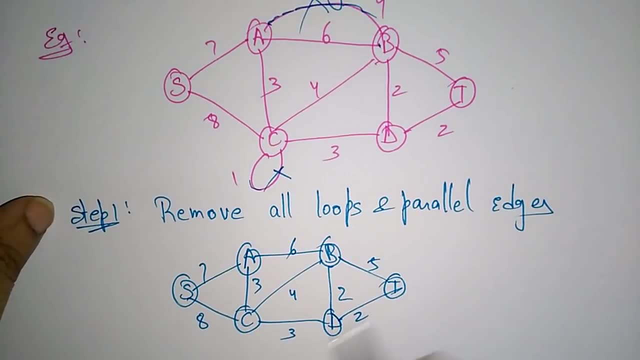 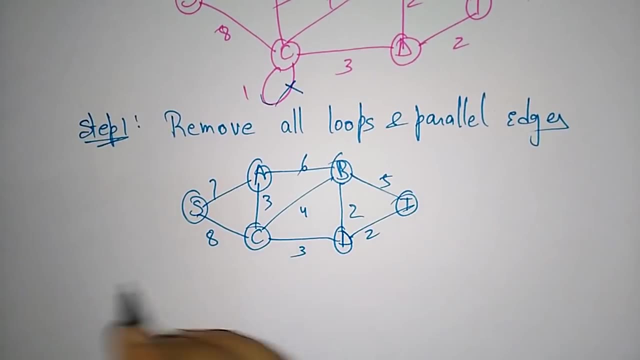 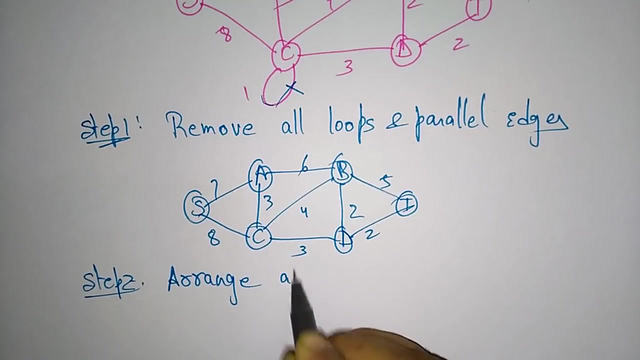 cost. So you just keep this 6 here and remove this 9.. So this is the loop. So I removed the loop and the parallel edges. Now coming to the second step. So in the second step, the algorithm for the second step is we have to arrange all edges, Step 2.. Arrange all edges in their increasing order of weight. 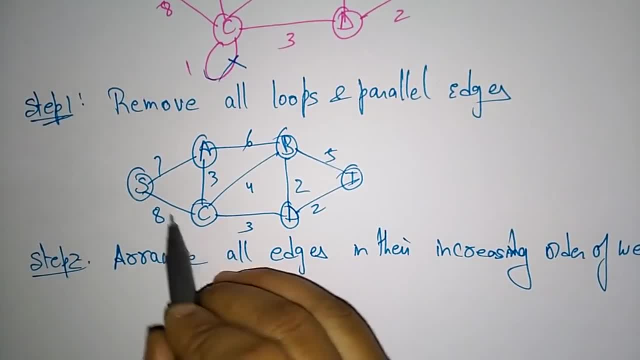 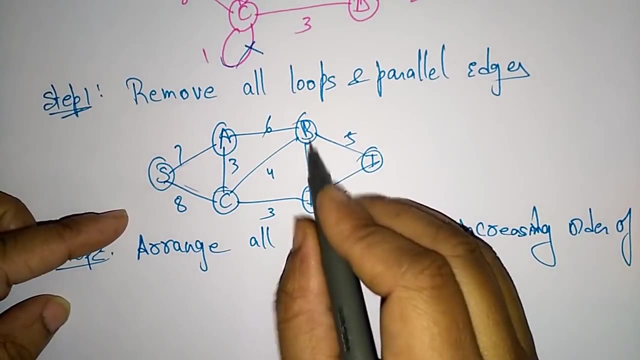 So I have to select, I have to arrange all the edges, whatever the edges. So these are the edges, These are the vertices and these are the edges. So I have to arrange all edges in their increasing order of weights. So what are the increasing order of weight? So first is 2.. So select B, D, So the weight is 2.. 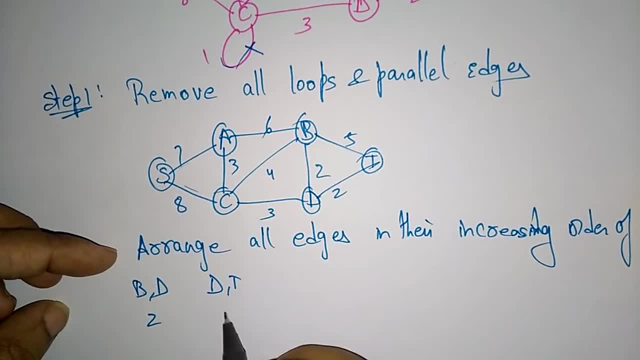 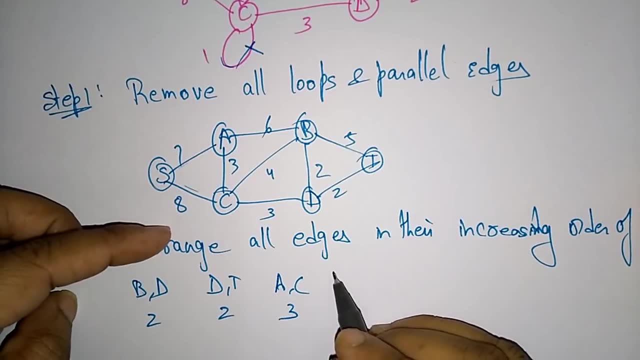 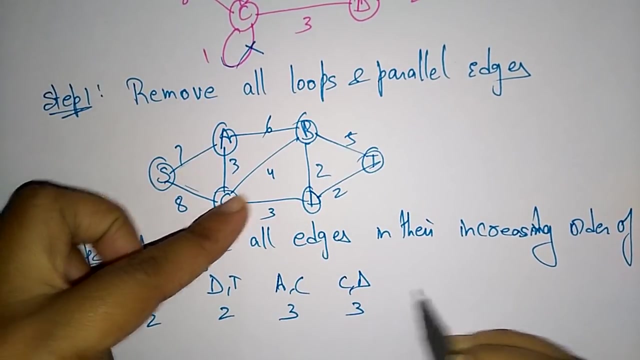 So next increasing order is D, T, D, T is 2.. Ok, And next is A, C, A, C is 3.. Next is C, B, C, D, C, D is having 3.. So C, D is 3.. Next is C, B, 4.. So after C, B, you are having: 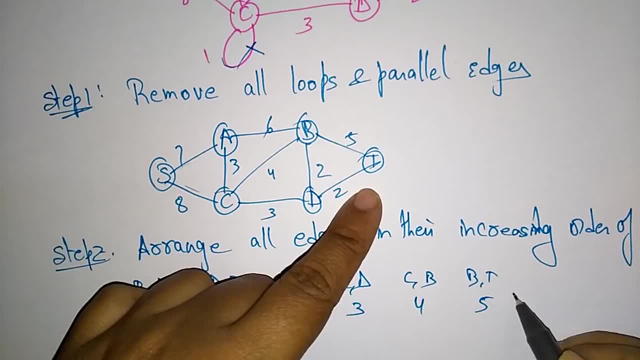 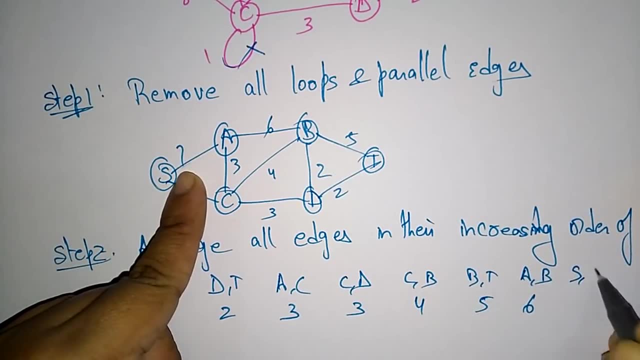 B, T, B, T is having 5.. Again, next is A B. Yeah, A B is having 6.. Next is S A, S A is having 7 and S C is having 8.. So now I arranged all the edges in their increasing order of weight. So I have to. 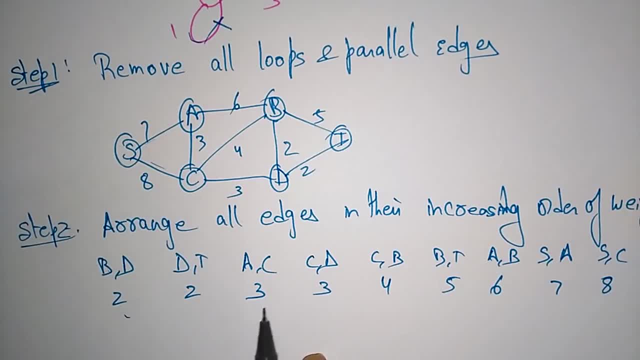 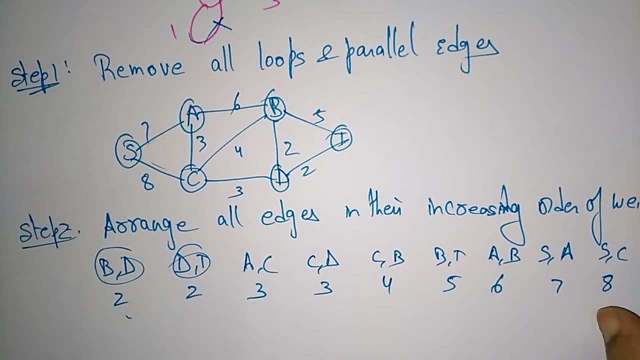 arrange all edges in their increasing order. First I take 2,, next 3,, next 4,, 5,, 6,, 7, 8.. So all edges. So these are the edges. So I arranged edges in increasing order. So that is the second. 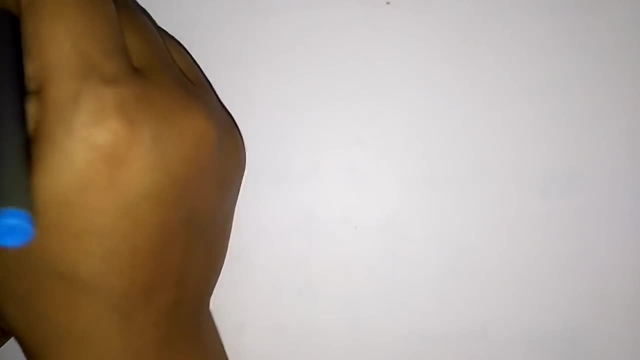 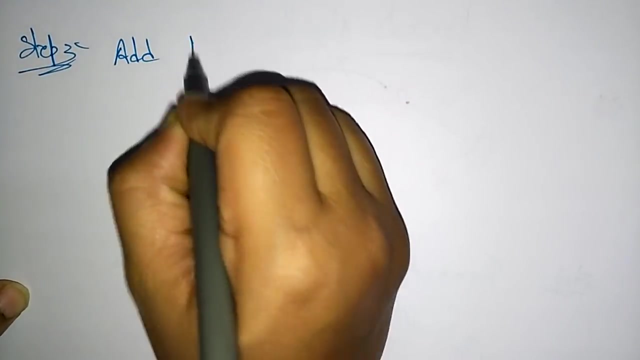 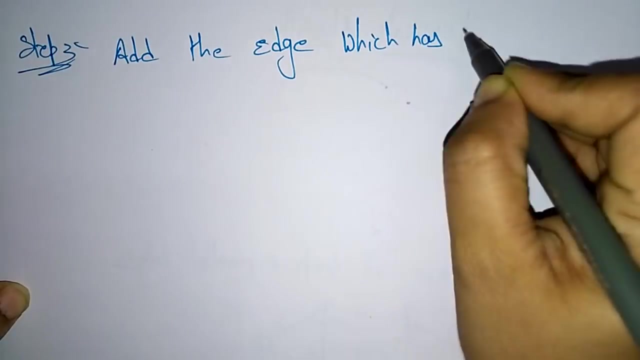 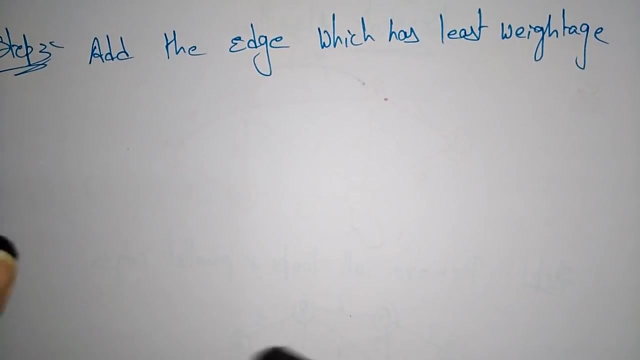 step in the algorithm. Now coming to the third step, What I have to do in this third step. So in the step 3, I have to add, add the edge. add the edge which has least weight. Least weight Least weight edge. I have to add the edge which has least weight Means. first I have to 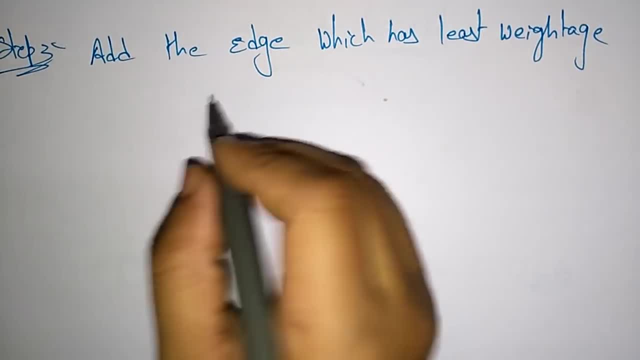 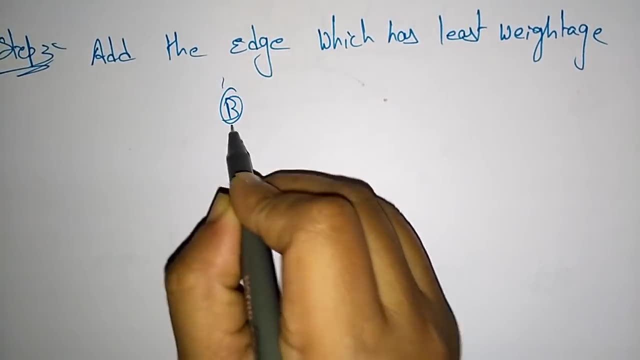 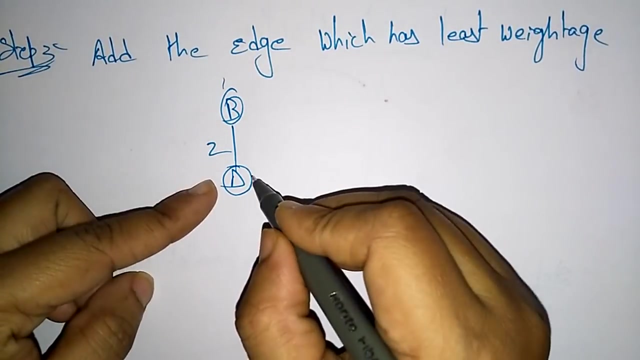 select the least weight, the starting, the. I arranged everything in the increasing order, So the first is the B D. B D is having the least weight as 2.. So I have to add the edge which has least weight edge. Next least weight edge is D. 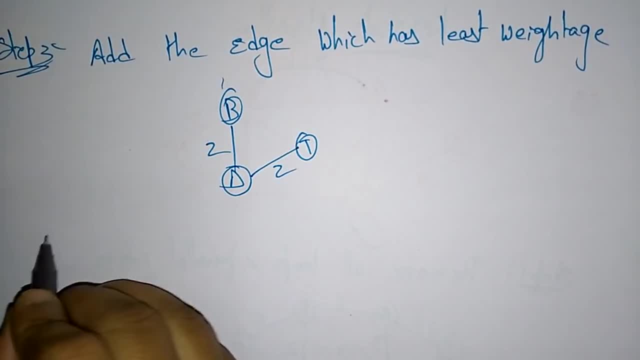 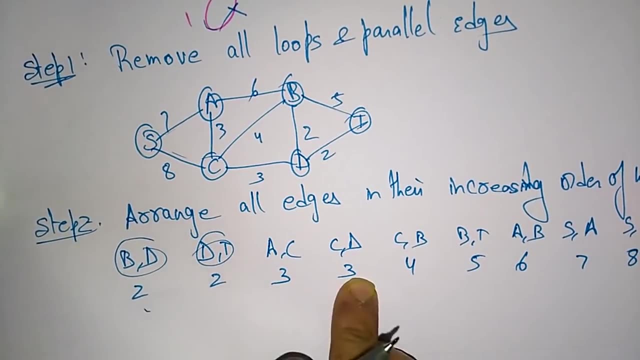 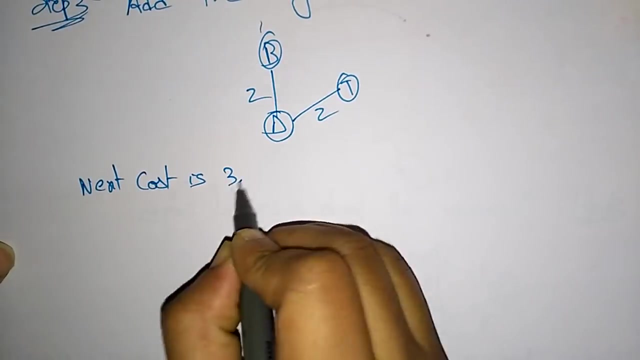 DT is having 2. T, So coming to the next cost is Okay. So here the next B D DT is over. Next cost is 3.. So 3, you are having 2 elements, 2 edges. Next cost is 3.. So the edges. 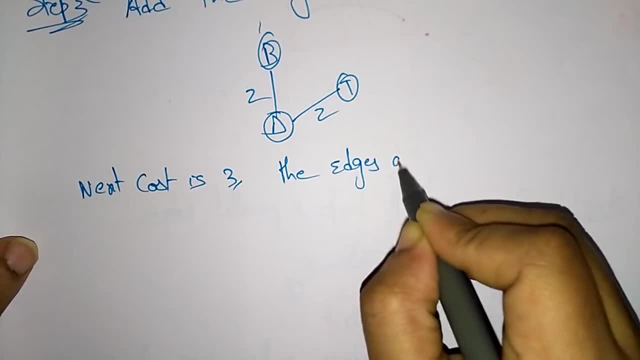 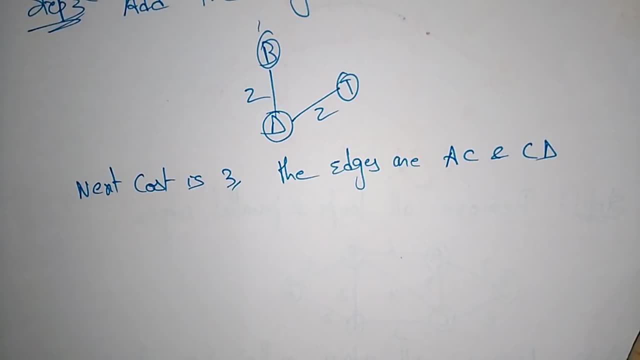 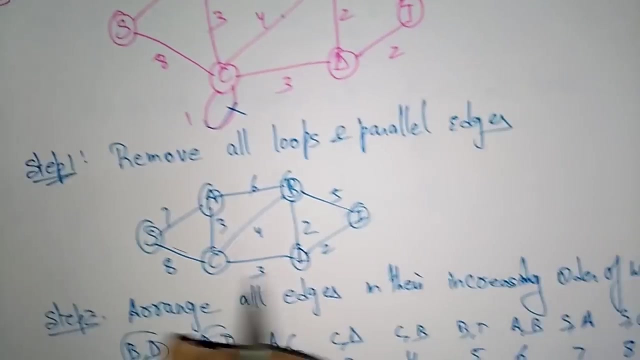 are. so the edges are A, C and C, D. So anything you can select A, C or D, So anything you can select A, C or D, So the edges, so the edges, CD. so I'm selecting AC, AC, CD and this is B and this is T. okay, so why I didn't? 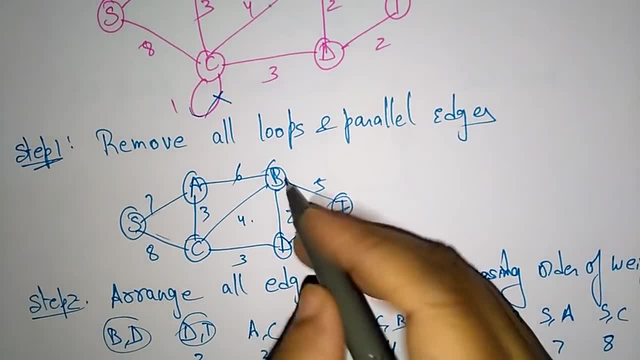 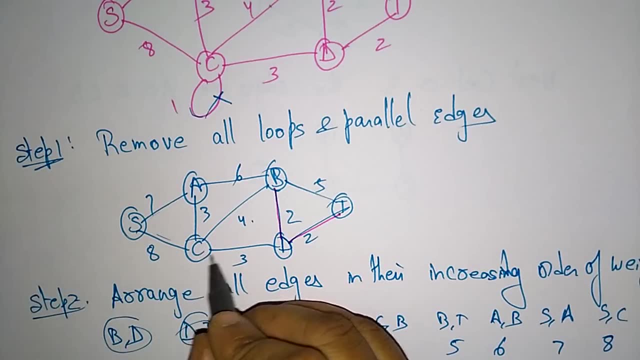 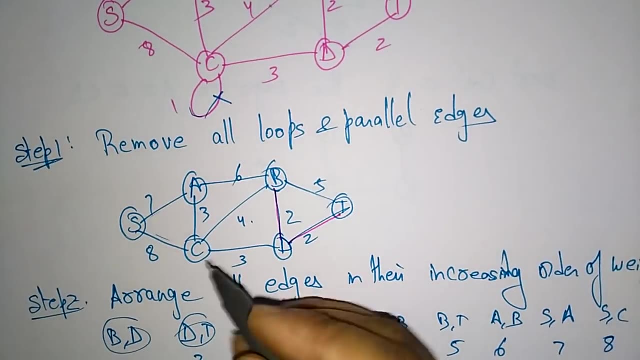 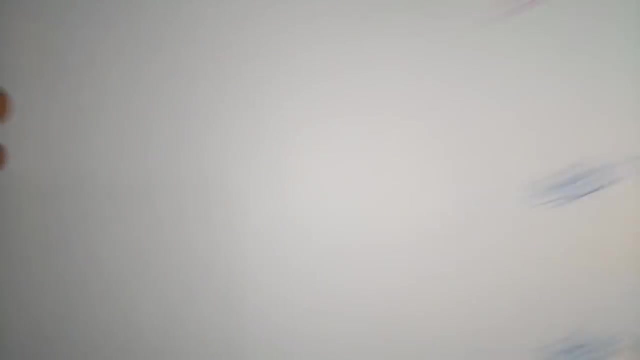 take the CD. I just only taken the AC. first I selected BD, least cost, and next is DT, next least cost. so it next is CD. I have to select either CD or means. next edges are AC and CD. so AC- both. I have selected AC and CD. okay, so the 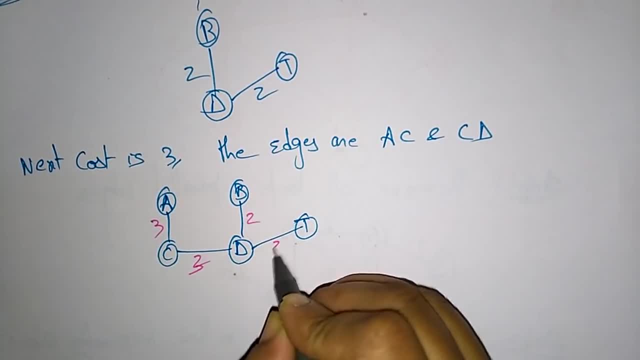 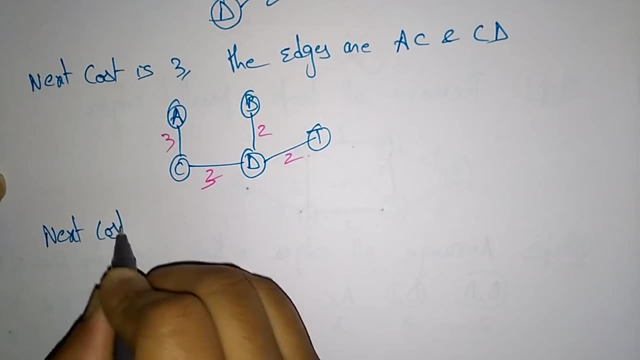 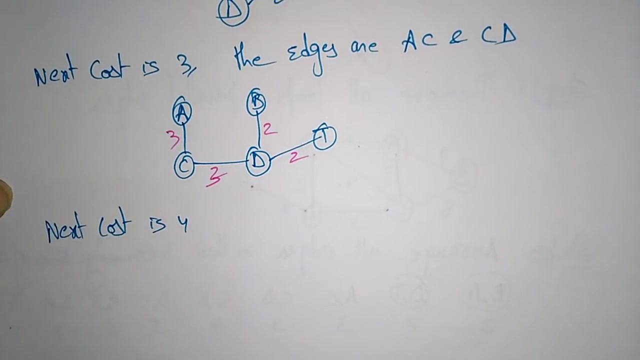 weights are 3, 2. sorry, 3 2, 2. so the cost 3 is over now. next cost is 4. so this kushkal's algorithm is mainly based on the edges. so we are this: calculate the minimum spanning tree based on the edges, so not focusing on. 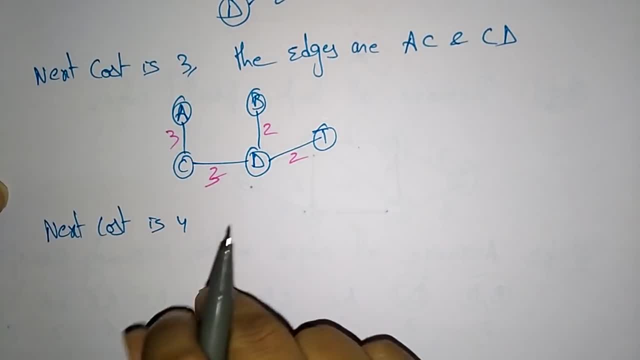 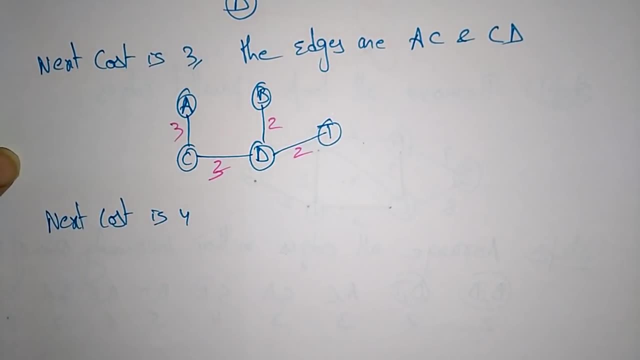 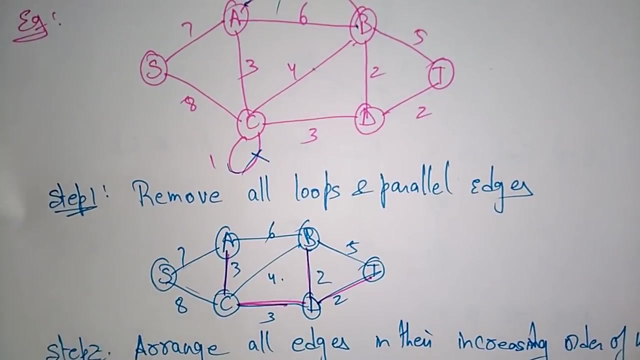 the vertex adjacent vertices of the visited vertex. but here we are focusing on the edges, with the cost increasing the least cost. so the next cost in the table is 4, but we observe that adding it will create a circuit in the graph. why it is creating a circuit in the graph, suppose if I select the 4? 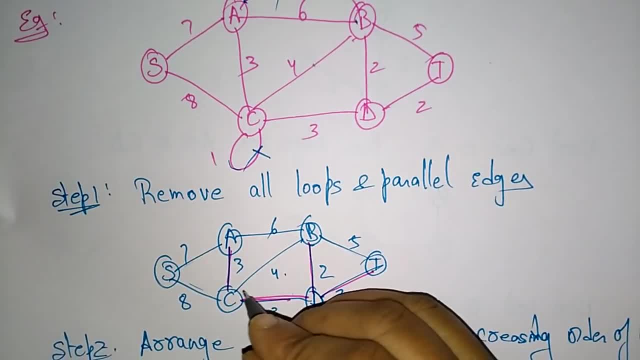 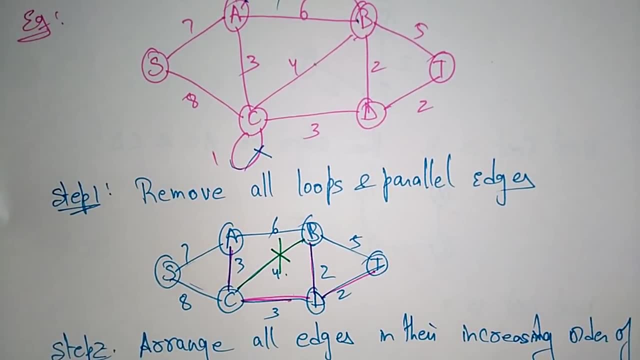 okay, if I select the 4 so it becomes closed circuit. so that's why I'm not selecting this 4, just discard it. so the main thing of the manning minimum spanning trees, you closed circuits are not allowed. so this see if I take CBA. 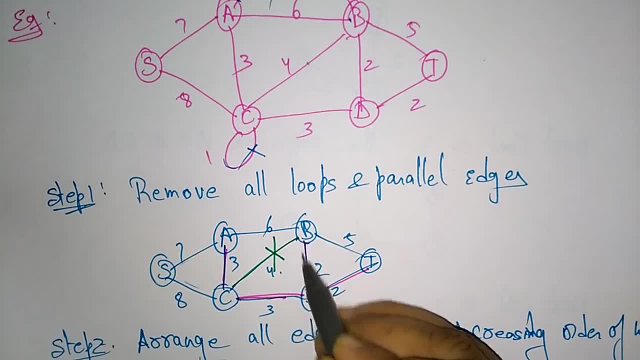 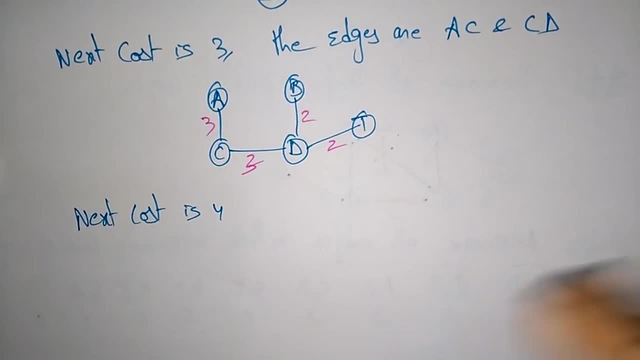 this: if I take this for, this becomes the closed circuit. so just discard this. 4. so we observe that adding it will create a circuit. that is a that in the graph, so we ignore it. in the process, we shall ignore or avoid all edges that create a. 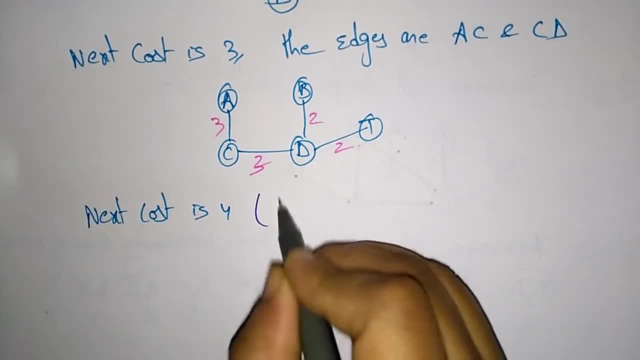 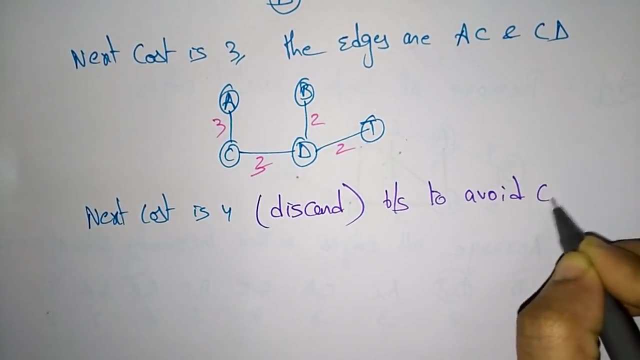 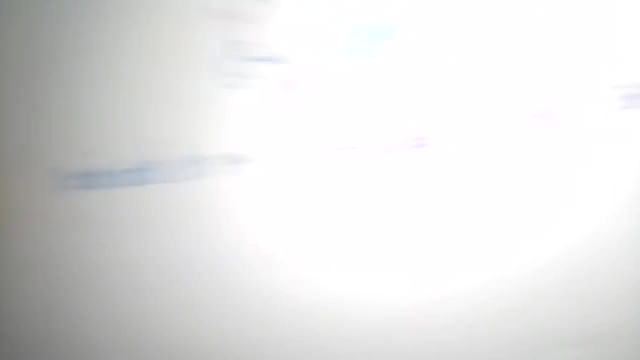 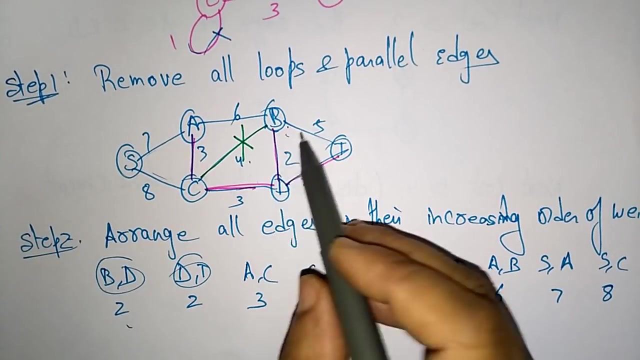 circuit. so whenever it creates a circuit you just discard it. discard because to avoid circuit. so next cost is I have to select the edges. after 4. what is the value? so after 4 that is a 5. so the fire I have to select. so if I select the 5, so 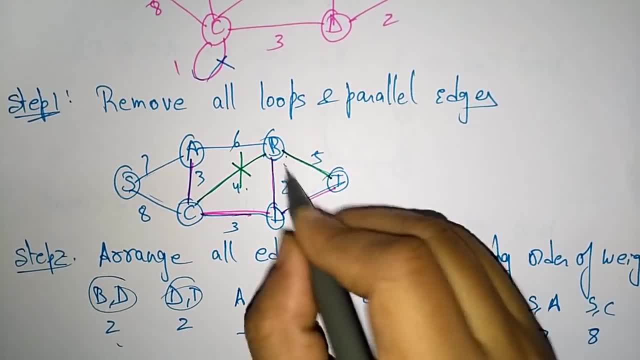 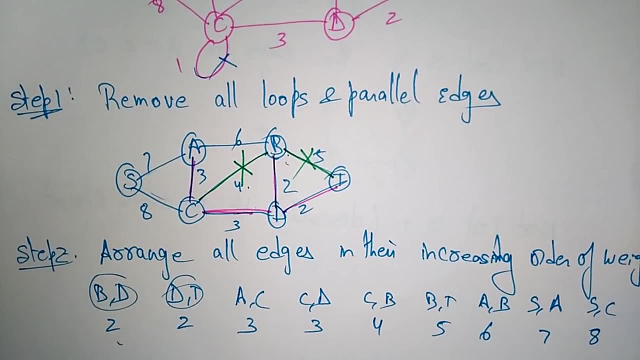 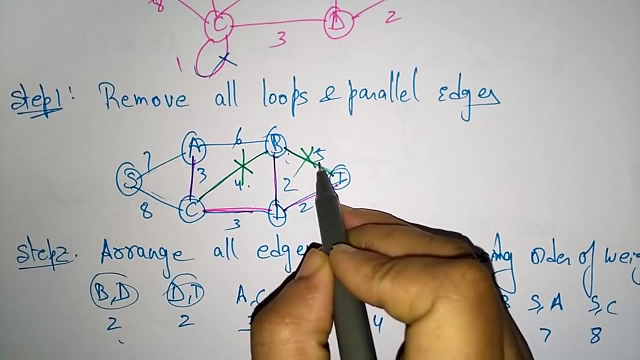 did you observe here? if I select the 5, it becomes a closed circuit. so just ignore this also. okay, so just ignore this also, suppose if I select 6, so the next cost of 5, after 5, the next is the. after 5, it is a 6, the next increasing. 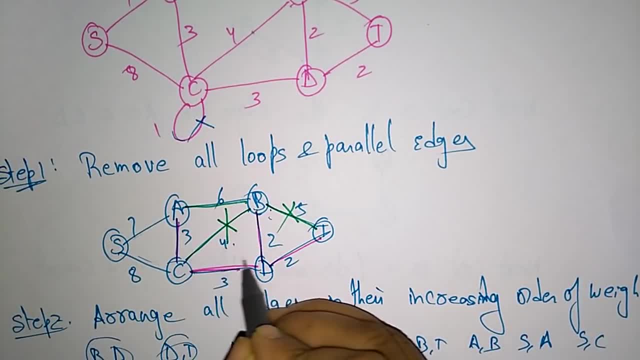 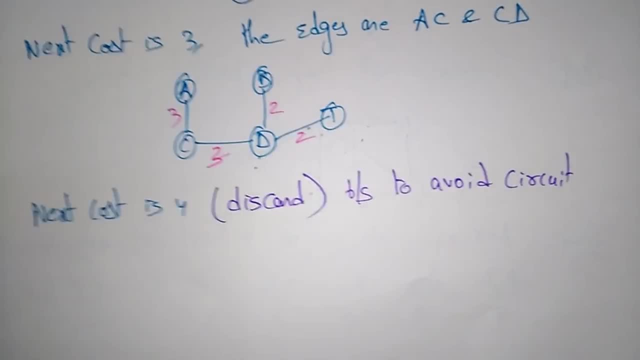 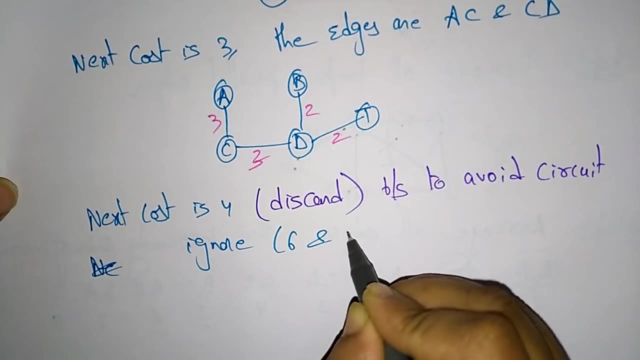 ses gone from 8, we have considered for 5. so the only progressive cost in this case will be 8. so if I choose 6, the closing weight is 6. so if I select six, this becomes closed circuit. so ignore this. 6 also the next stage we have to. 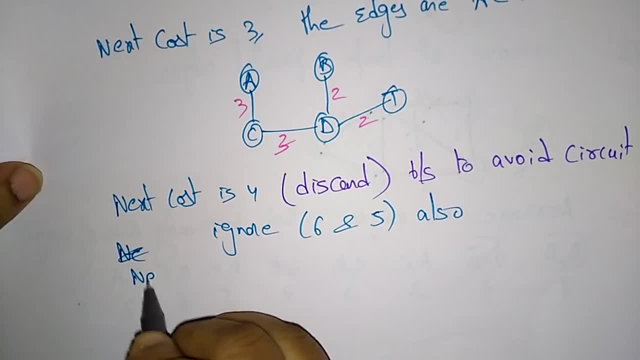 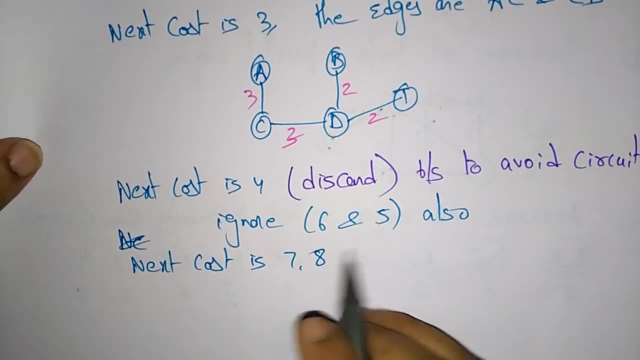 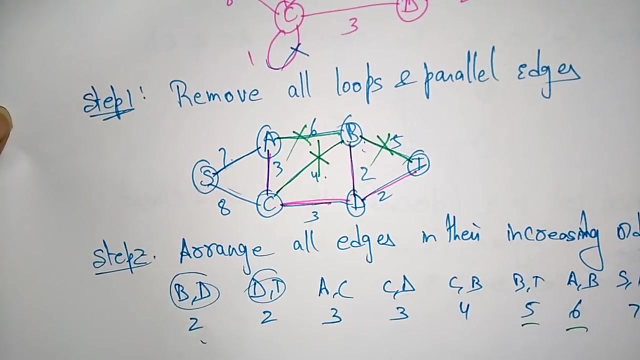 select is the, so we have to ignore 6 and 5 also cost. next cost: eh problem is 8, because we have to ignore this. took part in własng and eight, which is having the least least weight, that is a seven. so just select the seven. so now, 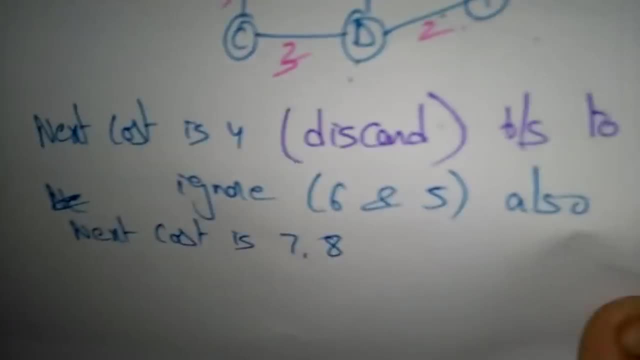 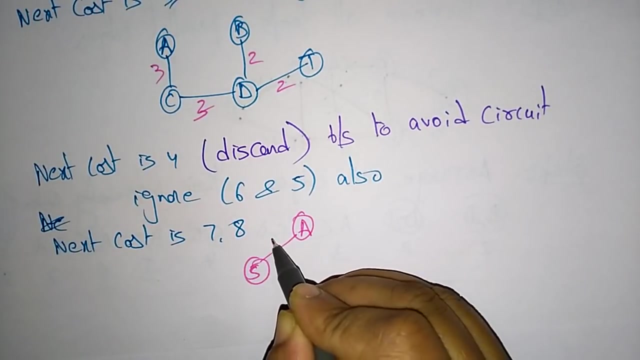 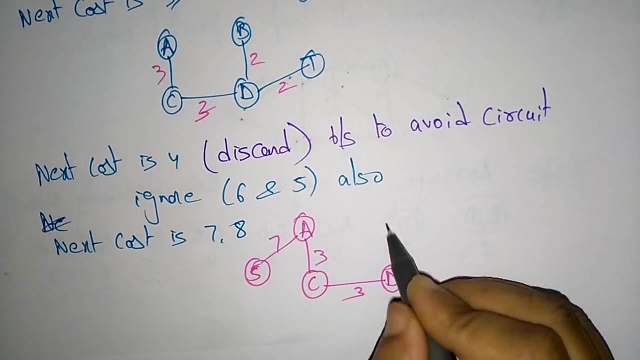 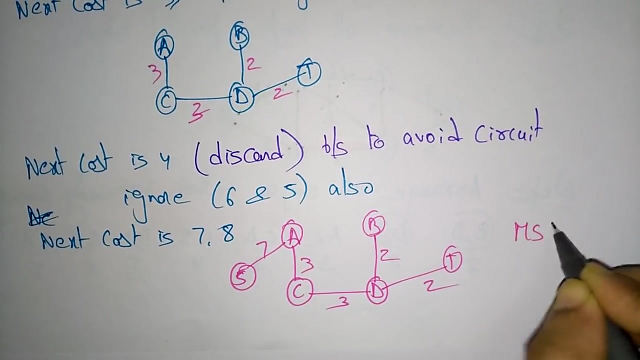 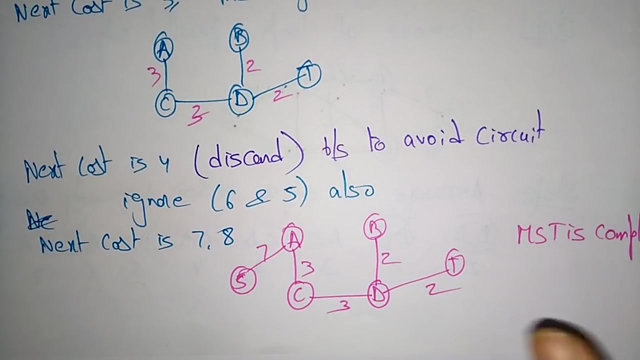 circuit becomes like this. so the final is a, s, this contains seven, c, this is three, d, this is three, and b, this is two, and t, this is two. so this is msd is completed. so this is how you have to calculate the kruskal's algorithm. so the only difference here, there and 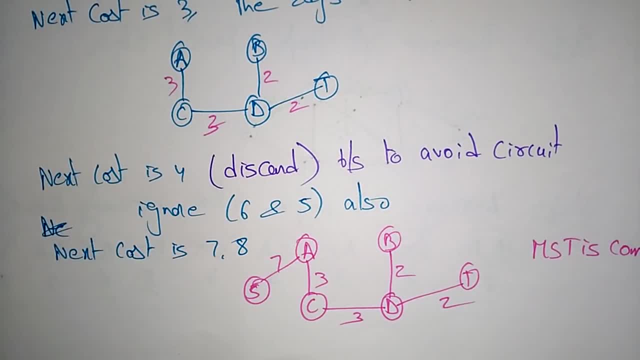 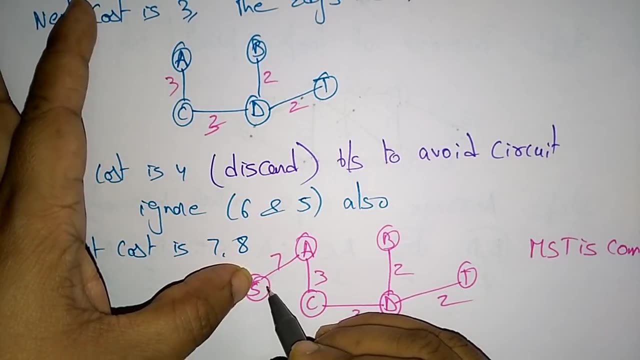 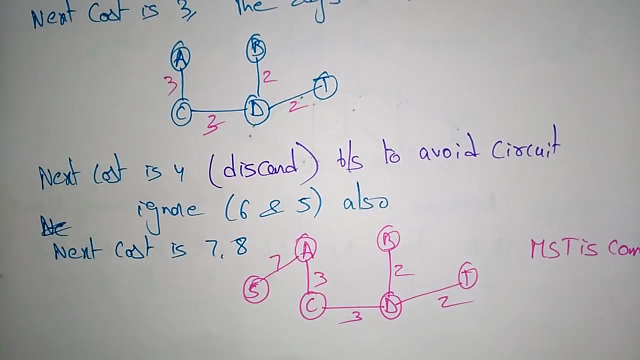 the kruskal's and the prince's. so there we are focused on the vertices and here we focus on the edges. so there you have to. in prince, you have to select only the adjacent vertices, which is having the minimum cost. but here, in edges, you have to first arrange all the edges in uh ascending order, uh least cost to. 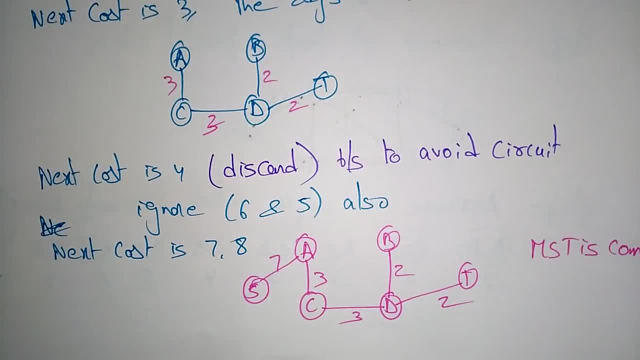 the highest cost. so first take the least cost and next select the least cost and observe for everything, whether it is forming the closed circuit or not. okay, if closed circuit is forming, just ignore that cost. so this is the kruskal's algorithm, thank you.